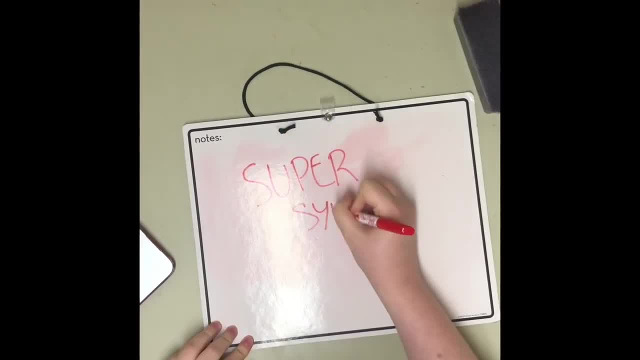 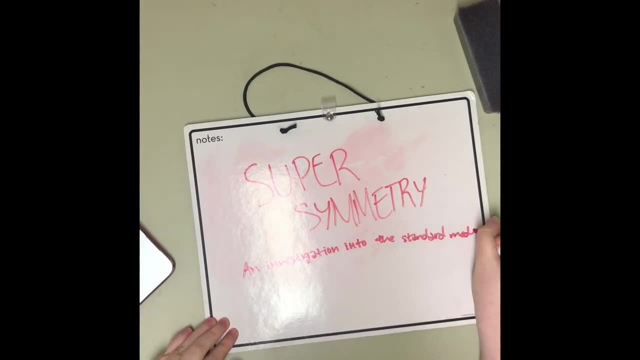 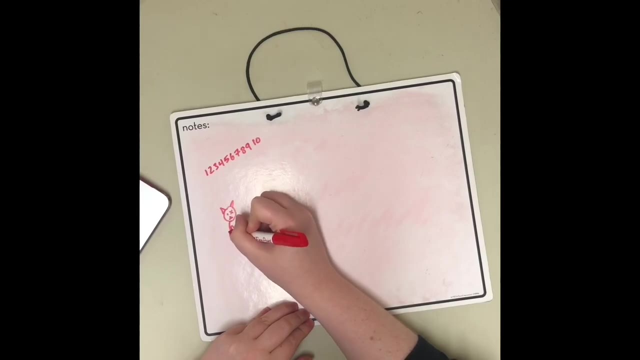 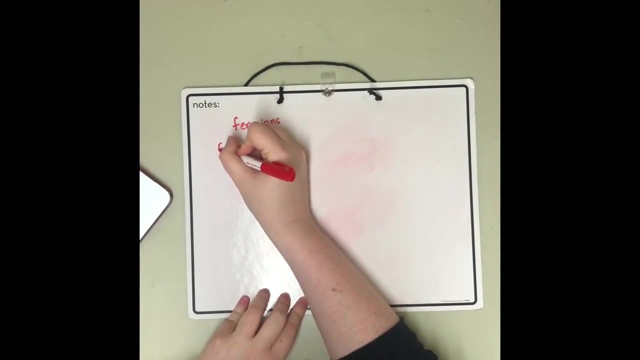 Shape or symmetry applies to a lot of fields such as math, quantum mechanics, condensed matter, for example. we've got optics, we've got string theory, we even have astronomy. but we want to focus today on particles. So let's first talk about the standard model. So we have in the standard model fermions and bosons. Fermions first are the particles that make up matter. They have spin- one half- and the spin is very important. We'll get back to spin in a second. Right now let's focus on what the actual particles are in the fermions. 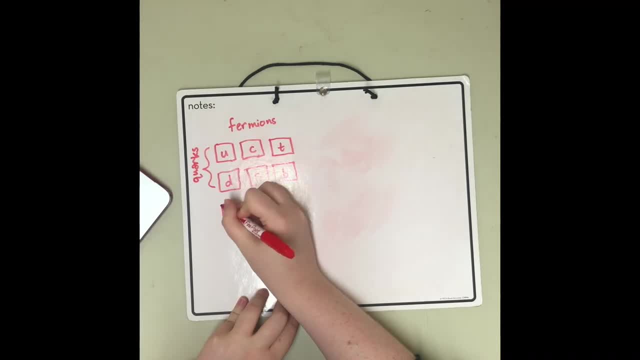 We have quarks first, and then we have the up-down quarks, the charms and strange quarks and the top and bottom quarks. Not a lot of creativity with these names. Meanwhile we have leptons, which include the electron, the muon and the tauon and their corresponding neutrinos. 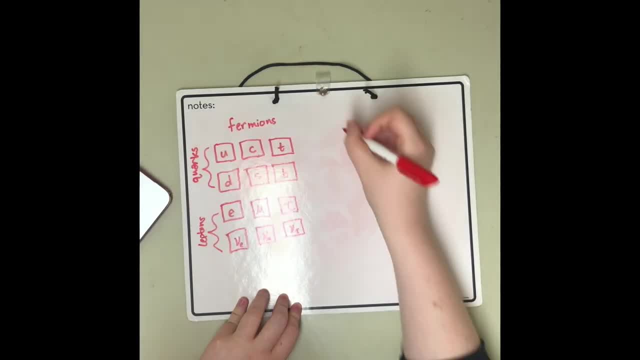 And so we. these, like I said, are the particles that make up matter that we see On the other side of the standard model, we have the bosons. These are the force-carrying particles. We've got the gluon, which is in charge of carrying the strong force. 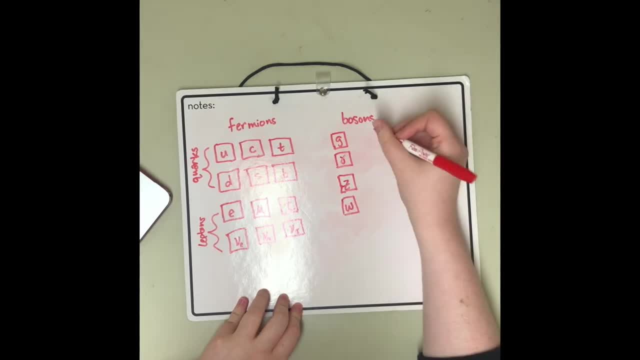 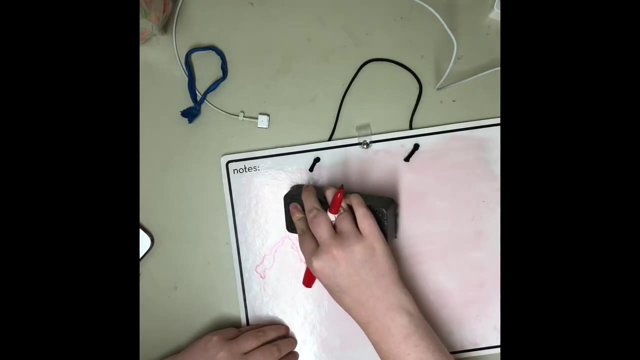 the photon which is in charge of after magnetic force, the z and w bosons which dictate the weak force, and the Higgs boson which gives all these particles the mass, or some of them. All right, so let's start talking about supersymmetry. Supersymmetry, or SUSSE if you will, is a way to connect. 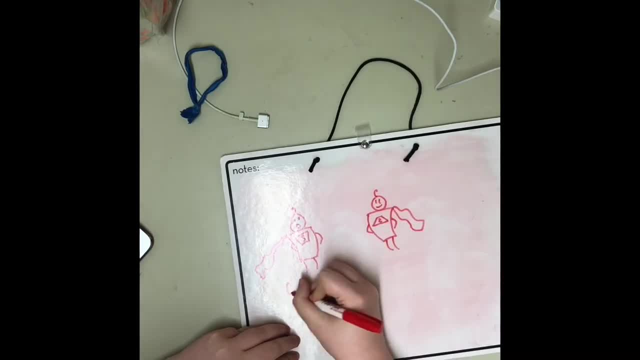 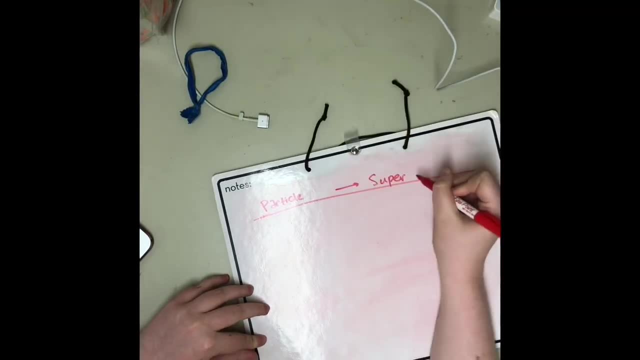 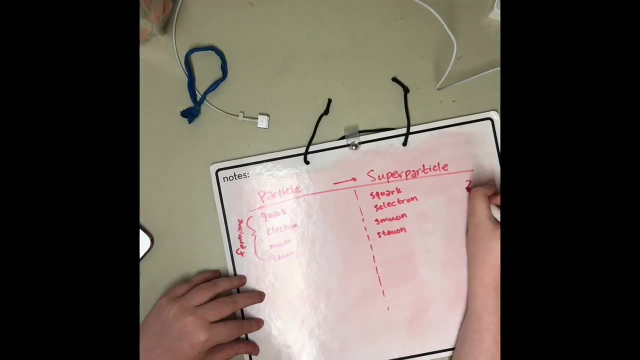 the standard model with some of the gaps that we haven't filled in yet. Basically, we make a partner particle for all the ones that I just listed. that changes ideally only in terms of the spin. So the fermions which have spin 1: 1⁄2, usually become bosons with an integer spin, and vice versa. 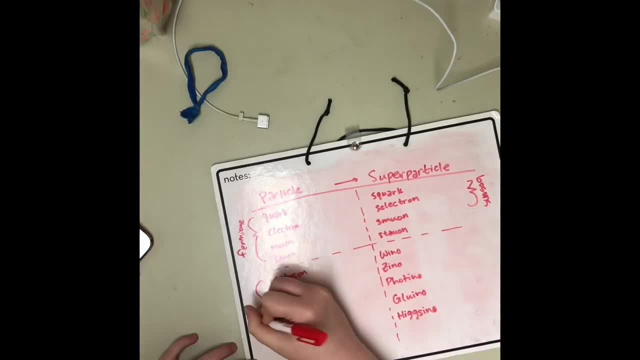 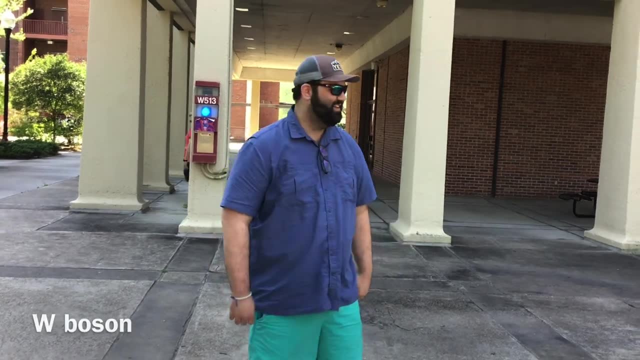 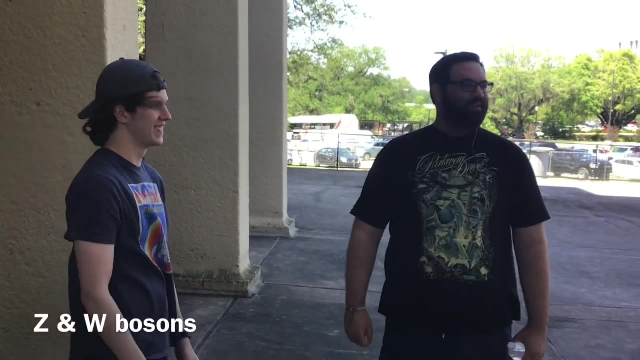 This simplification helps with a lot of equations that I don't yet understand. In the meantime, let's meet some particles, Alright? oh shit, Holy W boson. The W boson is capable of distorting another particle completely. It's friends with the z boson. the one…. 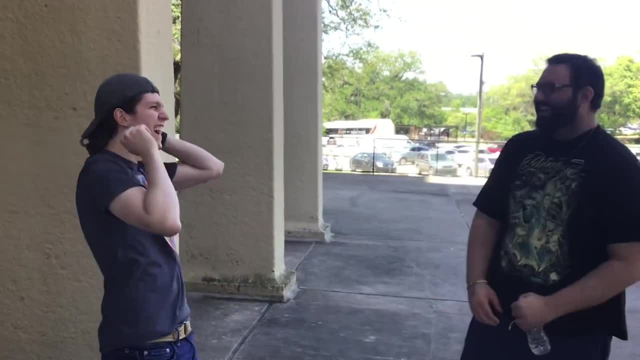 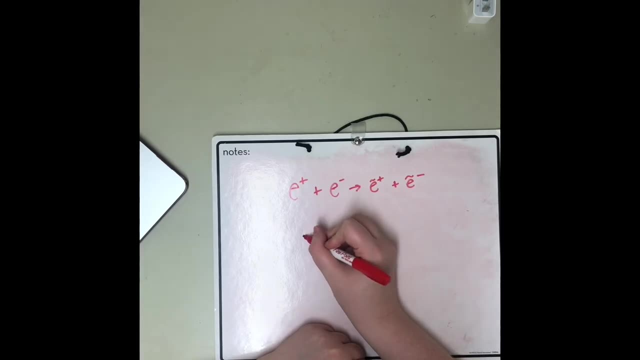 that carries the weak force with it. This weak force is incredibly strong compared to gravity in what's known as the hierarchy problem that we hope the minimal supersymmetric standard model might be able to explain. It's the simplest Sussie theory and cancels out a lot of the problems that 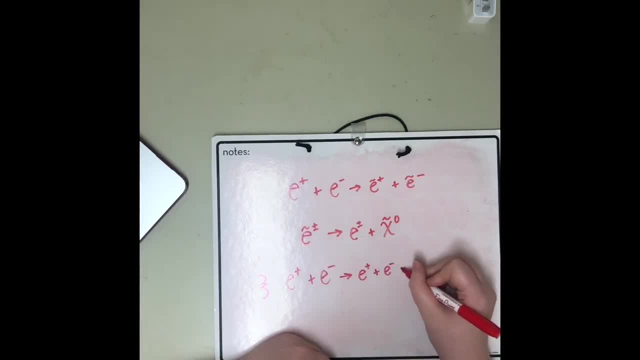 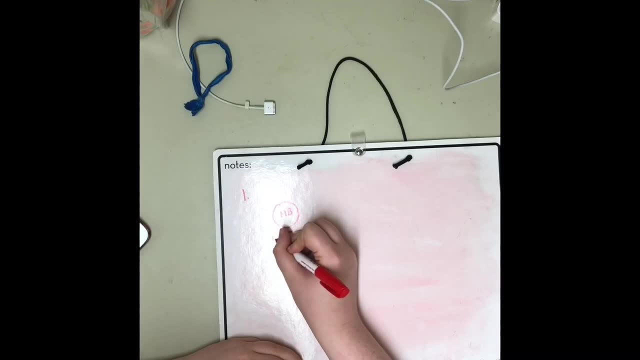 we have with hierarchy problems in the first place. Also, the equation on the board is a demonstration of how sparticles produce and decay in pairs. Sussie would help explain the huge mass discrepancy the Higgs boson has, because it's a lot lighter than expected and must give mass to W. 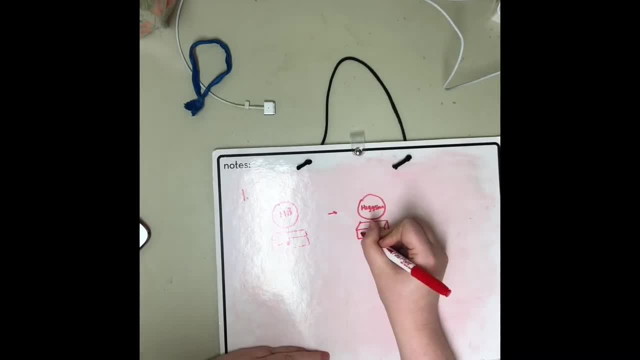 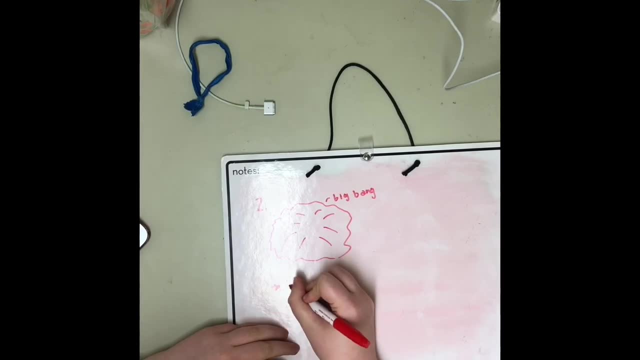 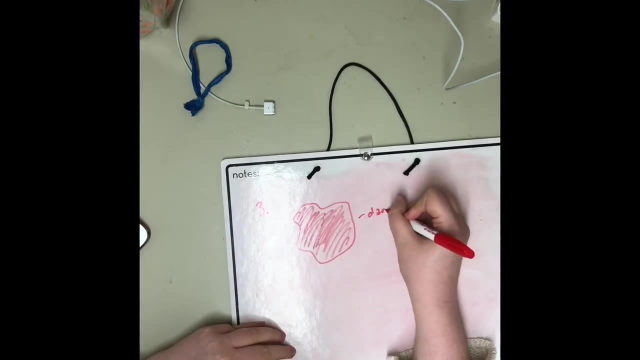 and Z. With the right Sussie equations, our gaps could be filled. Secondly, it could help prove the grand unification theory by making the strong, weak and electromagnetic forces have the same strength at high energies, just like in the Big Bang. Or it could be a dark matter candidate. 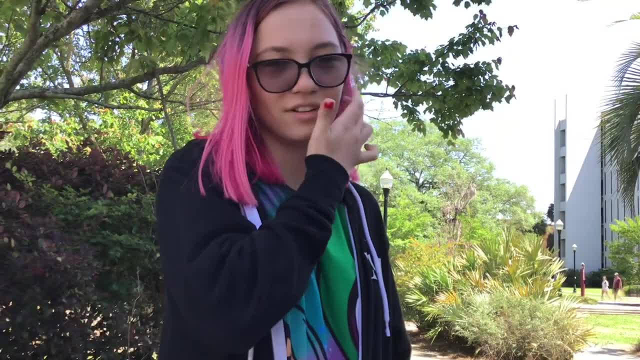 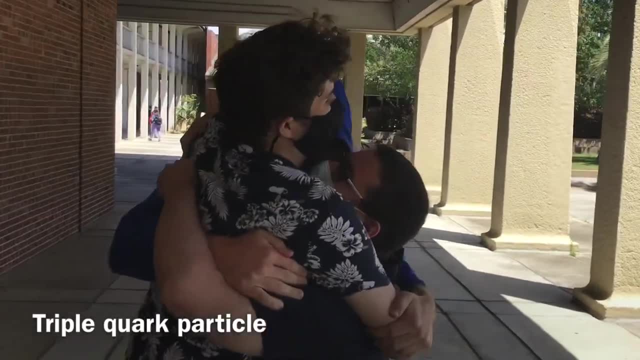 You yourself are a little bit negative, right? Um, yeah, you know I feel a little bit negative all the time, but I like to be around positive. These are three quarks. You don't ever see one of them in nature. They're a very social creature. 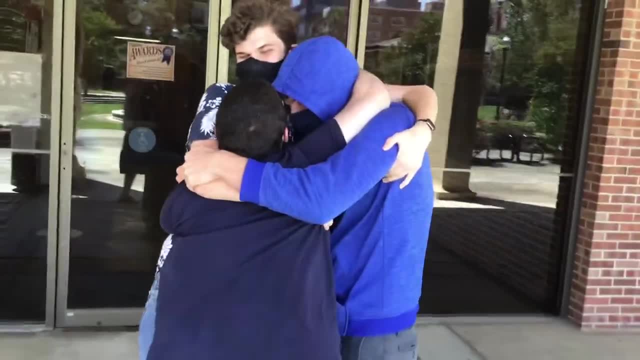 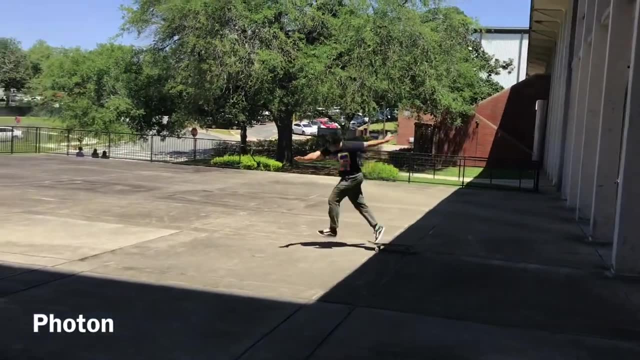 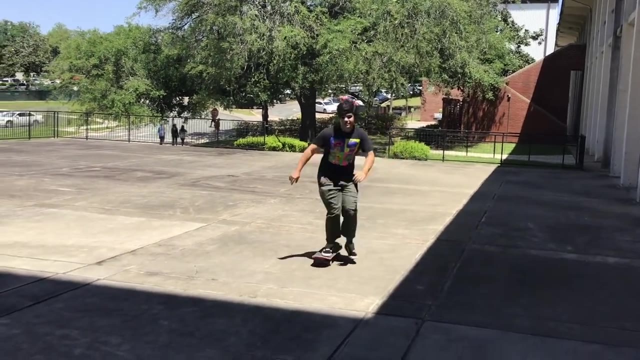 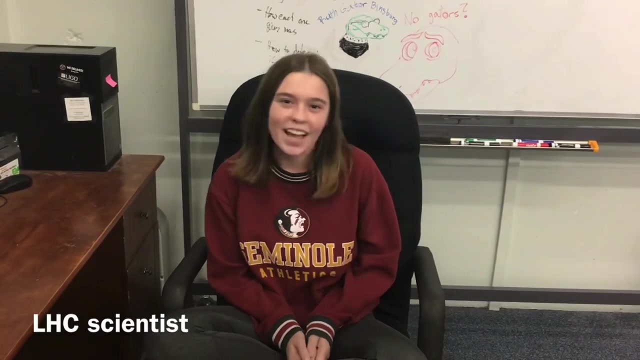 and the LHC has been unable to isolate a single quark. They comprise a ton of particles. This is a photon. He carries the electromagnetic force and if he goes fast enough then you can see him as light. I am a scientist. at the little LHC lab. I'm a little scientist and upon my discoveries I think. 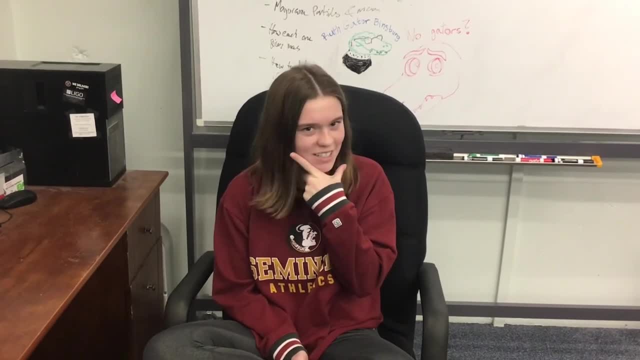 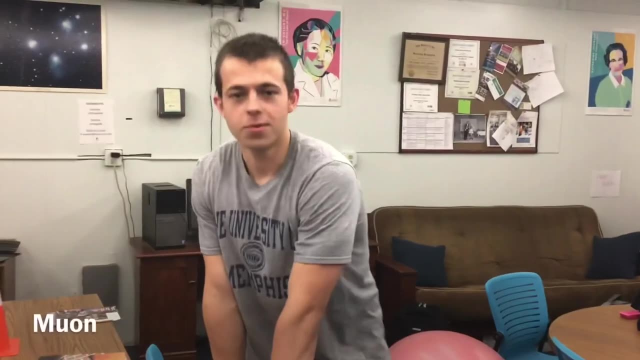 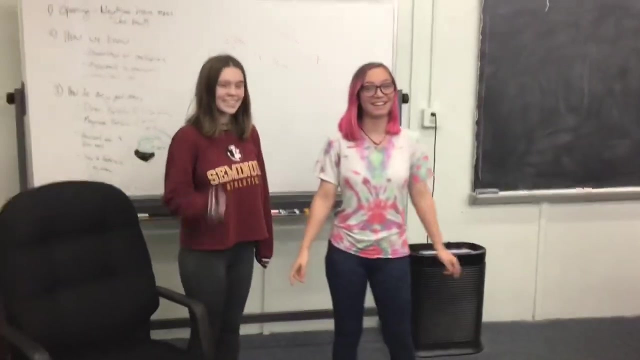 particles behave very interestingly. That girl with the red jacket on, I don't know. she keeps following me around and watching me. I'm freaking out, man, I don't know what to do. At the LHC, our scientist spins around an electron. 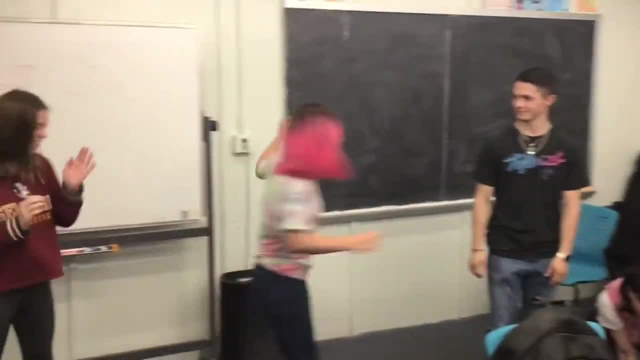 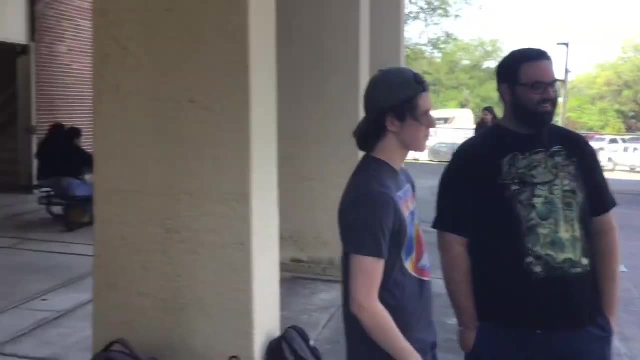 And once it's at a high enough speed, it will bump into another particle and hopefully make a Higgs boson. A Higgs boson enforces the connection between the weak and the electromagnetic force. I did that for the president. 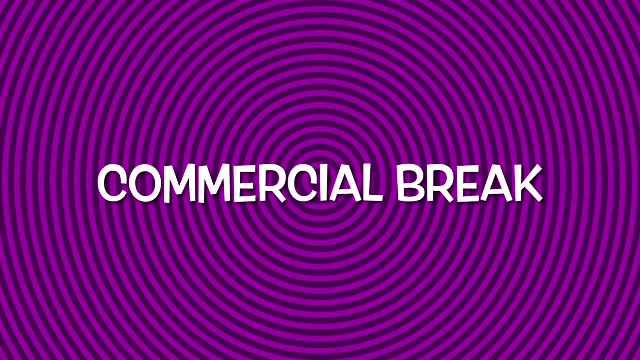 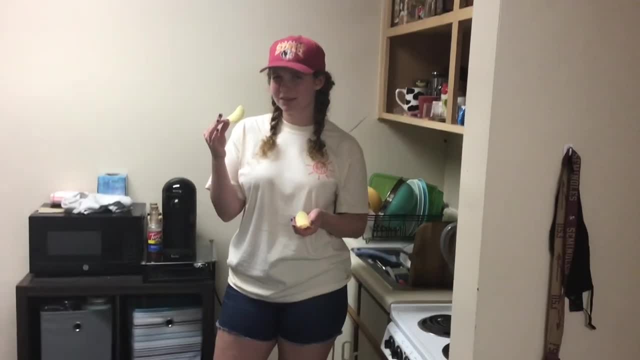 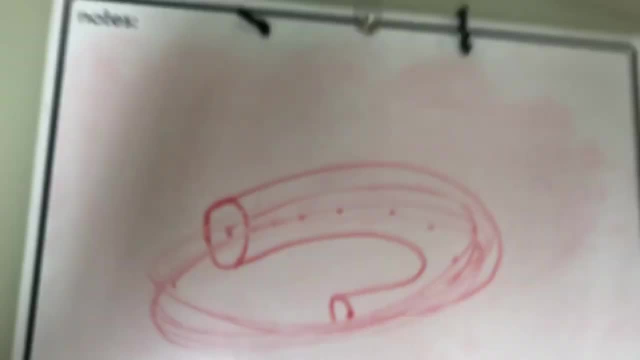 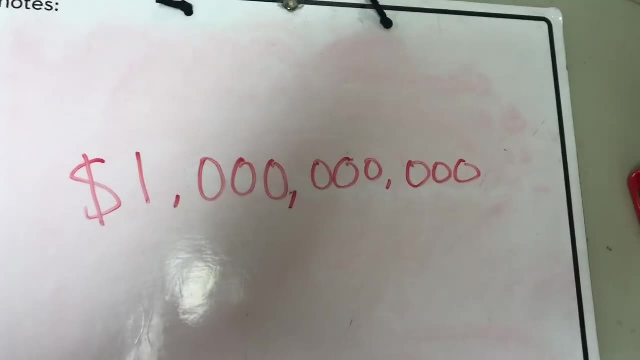 No, No, No. It speeds up particles round and round until it makes new things like this or this or even this, and you can have it at the low, low price of a billion dollars. Thanks, particle accelerator. Yeah. 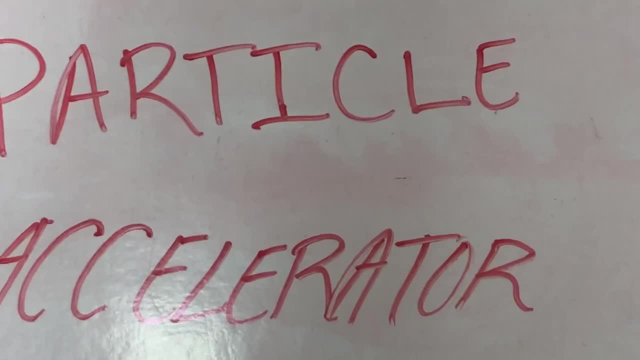 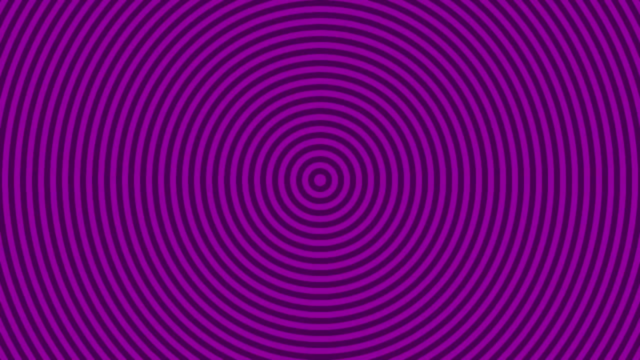 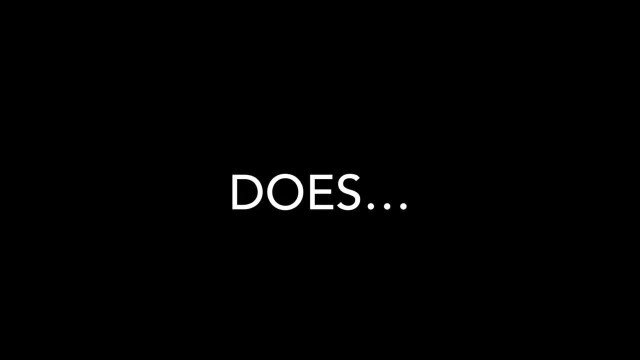 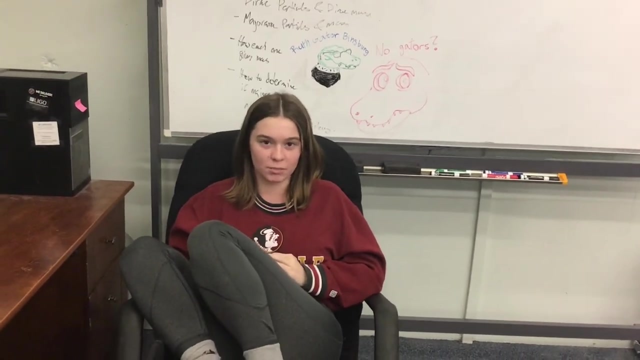 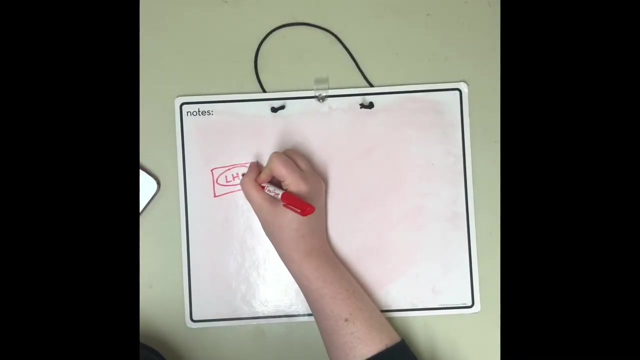 Particle accelerator does not come with batteries must be 18 years old to operate. Ah, Ah, Ah Ah. I don't believe there was enough evidence for supersymmetry, or else I would have seen it When the LHC was complete. scientists found the Higgs boson and felt really great about things. They were on the right track. the standard model was clicking into place and they figured for the last 40 years, as they had been theorizing that supersymmetry was right around the corner. However, as time went on, they didn't see any sussy particles, any sparticles. 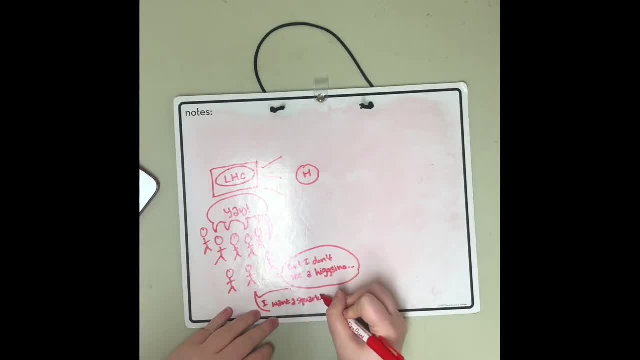 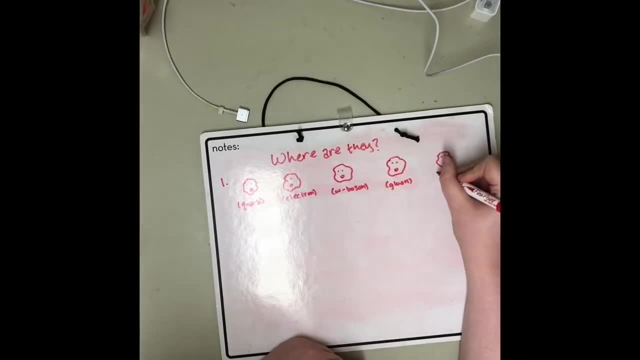 And so they kind of realized, oh, this isn't as easy as they thought it was going to be. And so some of the reasons that possibly, if sussy were to still exist, why we haven't seen it, is A these sparticles are actually much, much heavier than we think. 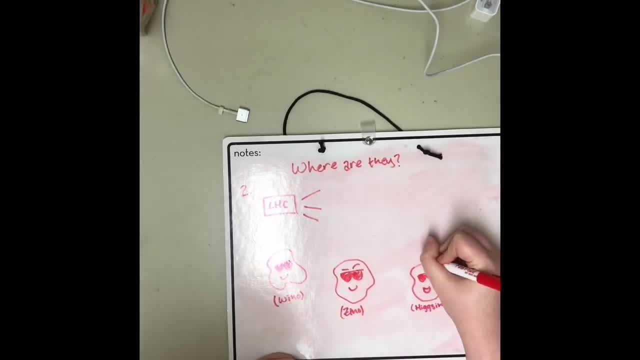 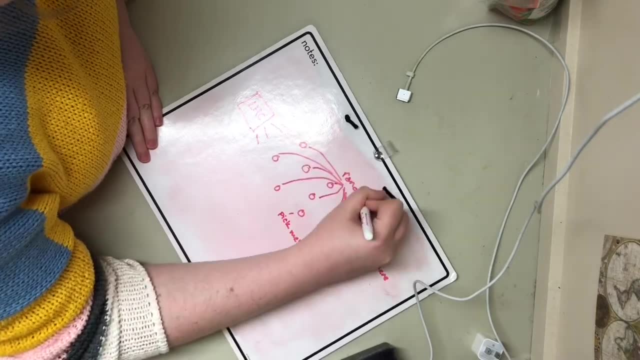 or B that we are unable to see them for one reason or another. Probably there is so much raw data that we're not paying attention to that. it might get lost. I'm the gluon Or not. for me, all those crazy porphyrs would be together. As a facilitator of the strong force. the gluon does indeed bind parts together to make particles. For a long time, scientists thought a gluina would be discovered, but unfortunately we have not seen one. Muons are much heavier than electrons, but still act similar to them. They come from cosmic rays and aren't made of quarks, and we believe that maybe the reason the magnetic field for it is stronger is because of nearby sparticles that pop in. So we haven't proven sussy to be true yet, but we're not ready to give up. 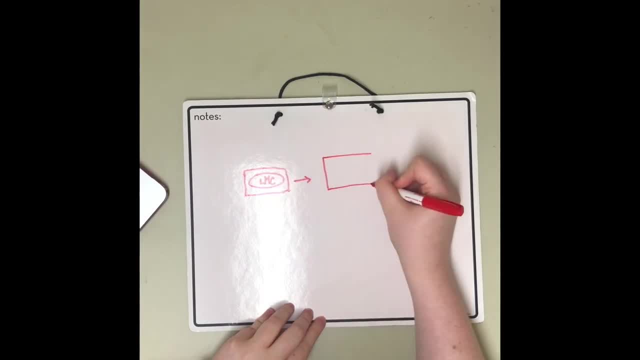 Let's say, if the sussy particles don't just difference but inextricably, and if it's actually that they are heavier as well, then with adjustments to the LHC over time and with lots of money we could see a sparticle.